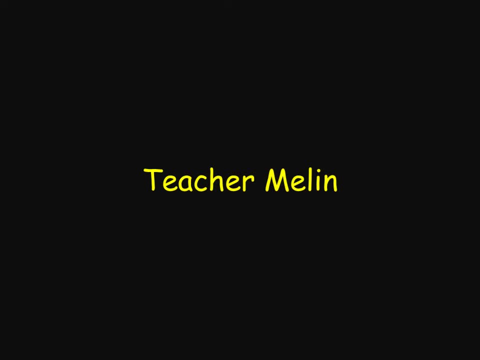 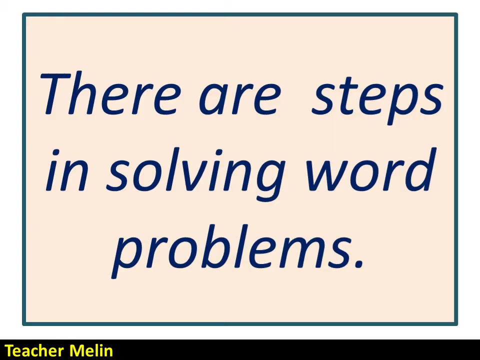 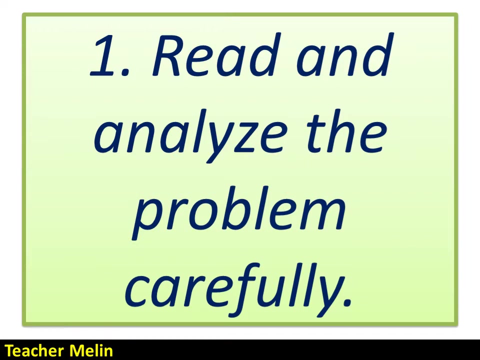 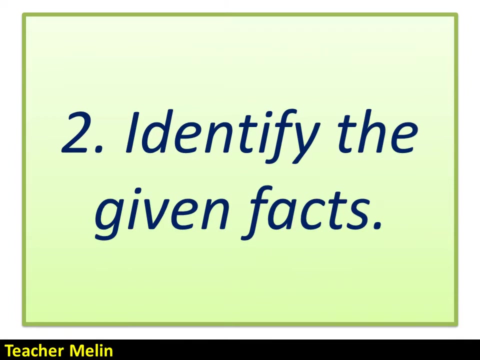 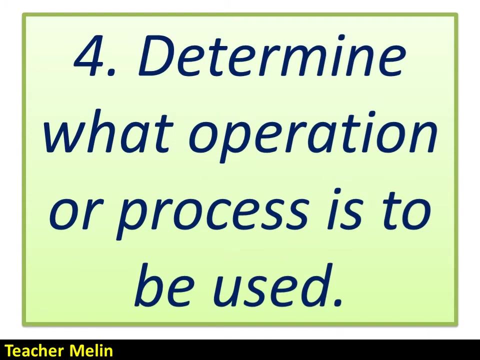 Problem Solving Involving Subtraction. There are steps in solving word problems: 1. Read and analyze the problem carefully. 2. Identify the given facts. 3. Identify what is being asked. 4. Determine what operation or process is to be used. 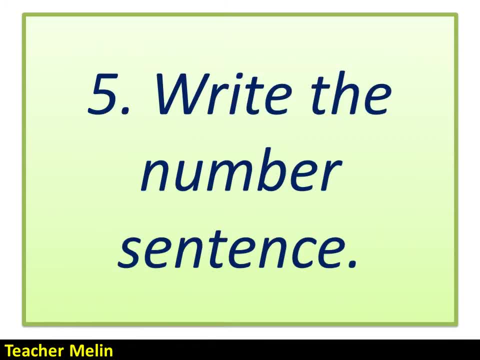 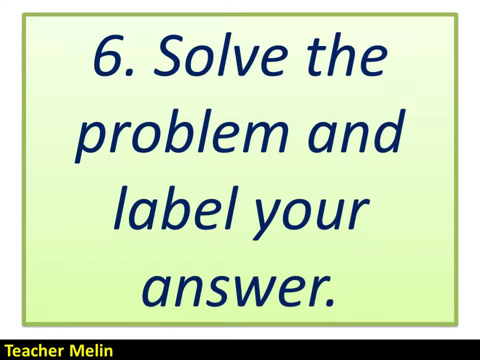 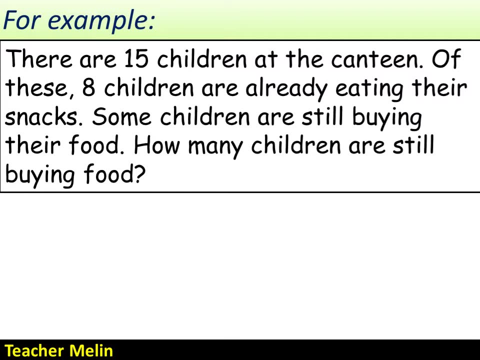 5. Write the number sentence. 6. Solve the problem and label your answer. 7. Write the answer. 8. Write the answer. For example, There are 15 children at the canteen. Of these, 8 children are already eating their snacks. 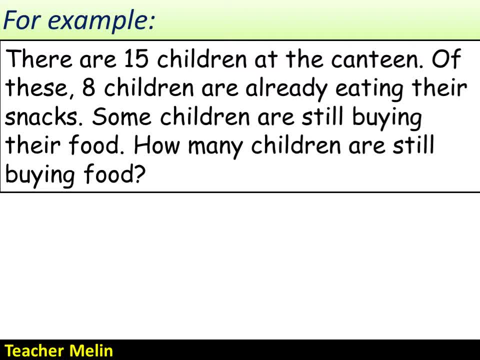 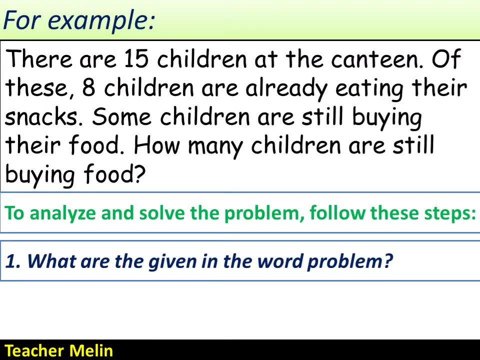 Some children are still buying their food. How many children are still buying food? To analyze and solve the problem, follow these steps: 1. What are the given in the word problem? The answer is: 15 children at the canteen and 8 children eating. 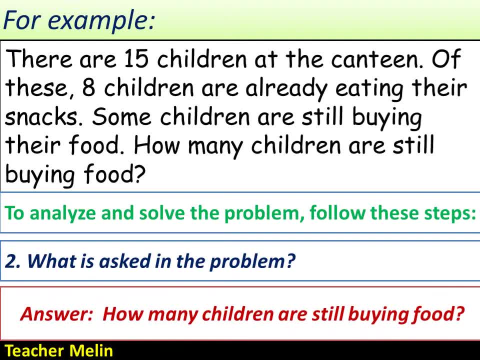 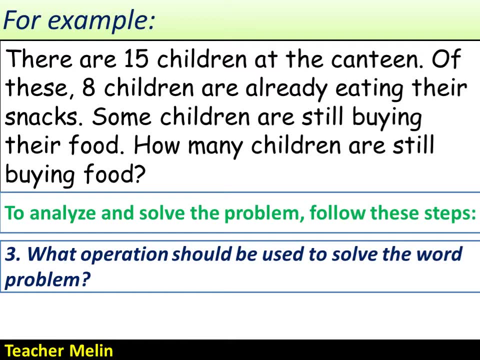 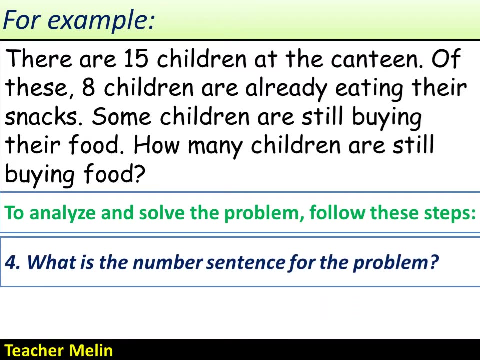 2. What is asked in the problem? The answer is: How many children are still buying food. 3. What operation should be used to solve the word problem? The answer is Subtraction. 4. What is the number sentence for the problem? 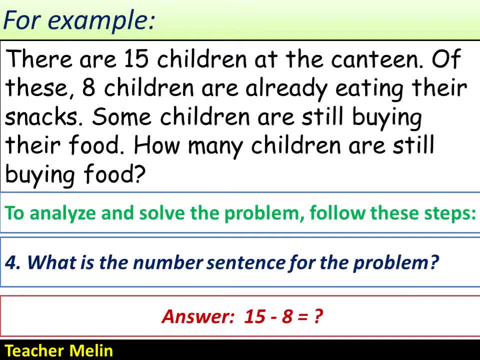 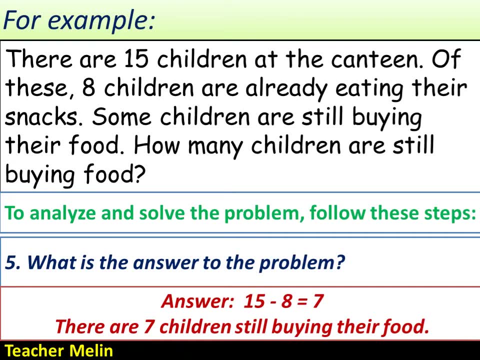 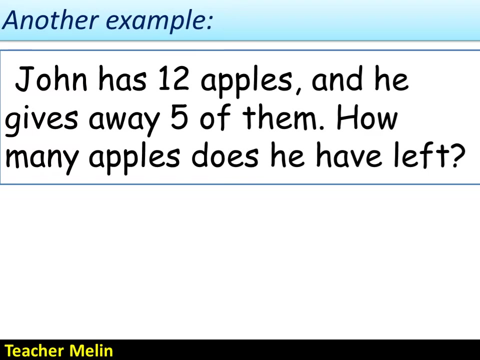 The answer is 15-8- 5.. What is the answer to the problem? The answer is 15-8 7. There are 7 children still buying their food. Another example: John has 12 apples and he gives away 5 of them.